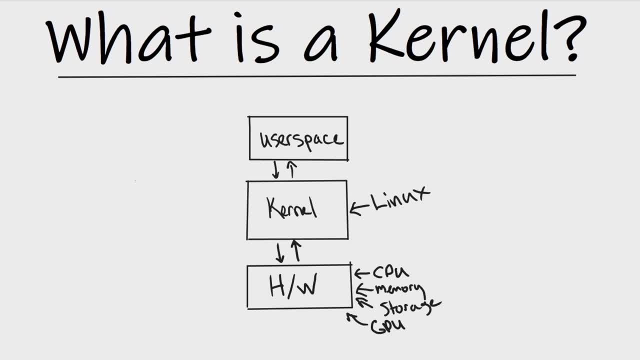 that's exactly what Linux is. A kernel is not an operating system. Instead, it's this program layer that we've been talking about, right in between the user space and hardware. Many people get that confused: when talking about Linux, They're actually talking about the kernel, But when we talk about Linux distributions, 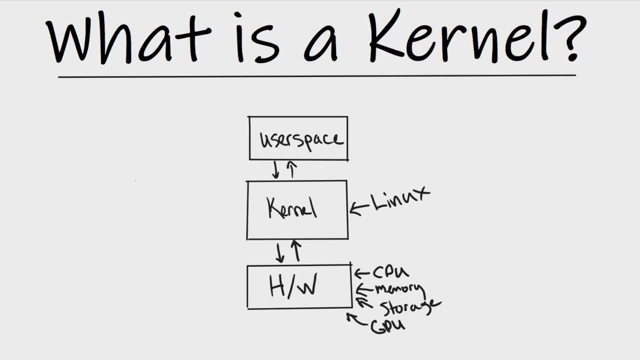 we're talking about packages that have been put together, For example a graphical user interface or desktop environment, along with many different programs and the kernel, different types of init systems. Those all go into making an operating system And then, of course, with those, Linux. 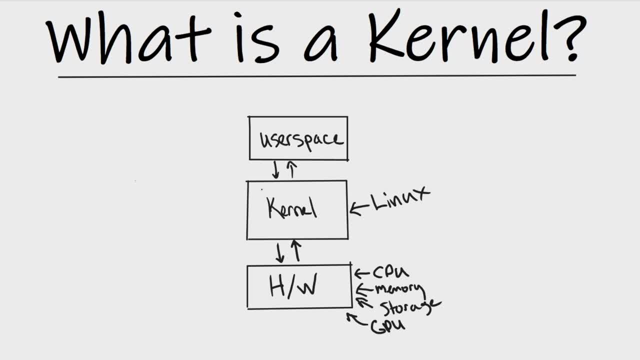 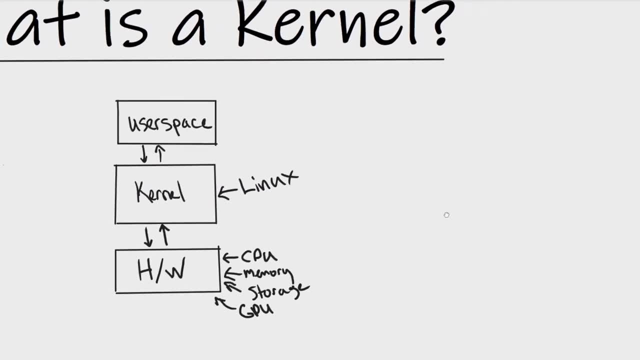 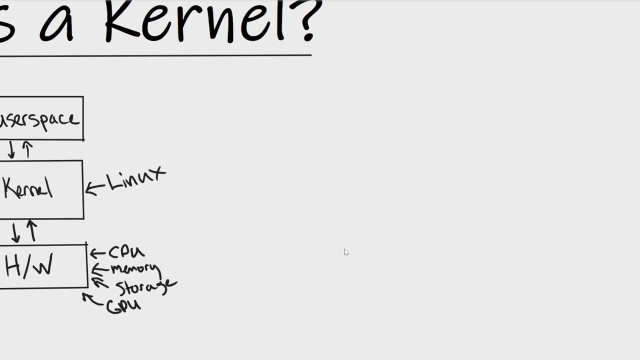 distributions. they use the layer of the kernel, or what's called Linux, to talk between the user's hardware, since it's already developed and very mature. So let's step aside and check out what the kernel actually manages. We spoke a little bit about the different layers, but let's talk 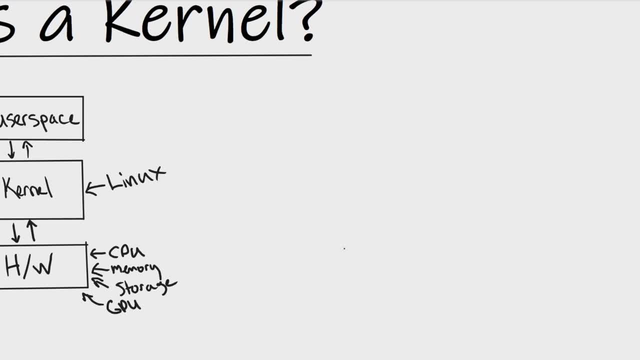 specifically about the kernel layer. So if we write out manage, let's talk about some things that it does manage. One thing that we already discussed is the CPU and its tasks that it's currently running. It helps translate and give instructions to the CPU in a format that it's. 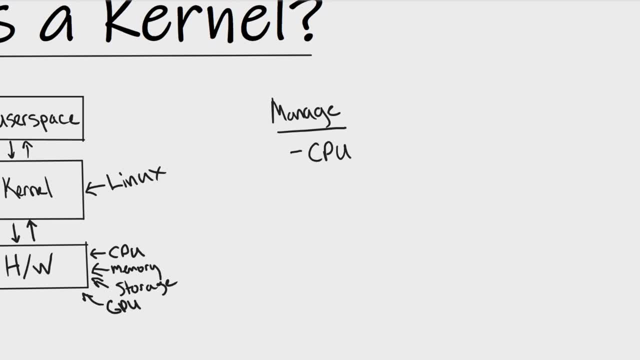 able to understand so it can process your information properly. Also, the kernel manages reading and writing out input and output devices. Another thing is scheduling, to make sure your system doesn't get bogged down and that it's properly taking care of tasks. It also takes. 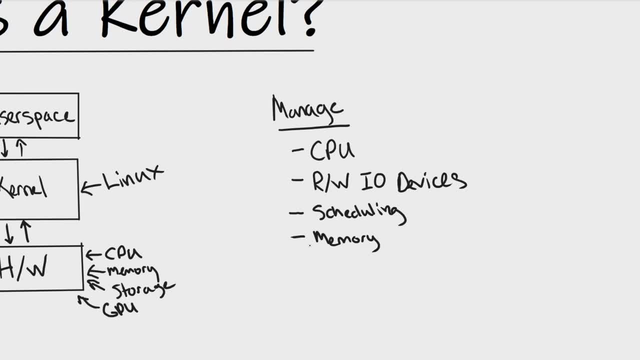 care of memory allocation and deallocation, cleaning up your memory as things open and close, requesting those resources as well as giving them back. Then another thing it does is it has some security built. in That way, programs don't cross together and are properly managed, because you wouldn't want to reach a space of another program. 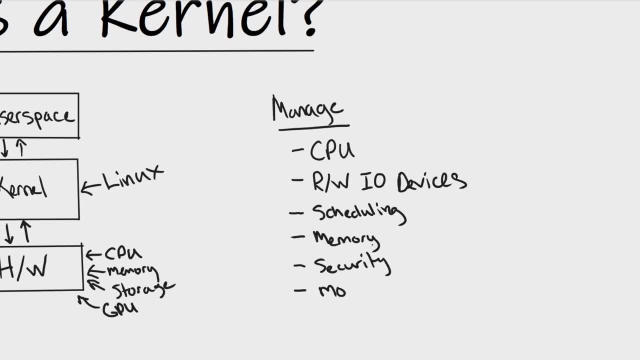 because that could create a security risk. Finally, there's, of course, more things that the kernel does. This is a really small list compared to everything that it does. A kernel is a very large piece of software. Back to the reading and writing of the IO devices. 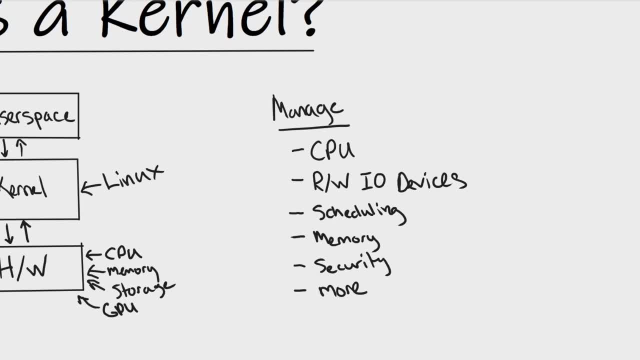 you can imagine, there's plenty of devices on your computer: Computers such as a storage disk, CD-ROMs, USBs, all that fun stuff which require drivers to talk back and forth user space, and hardware, which of course exists in the kernel as drivers, and 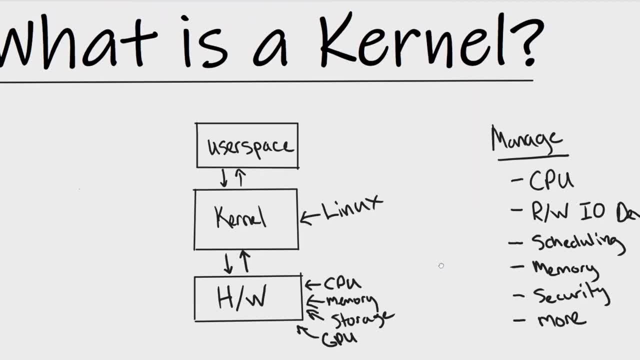 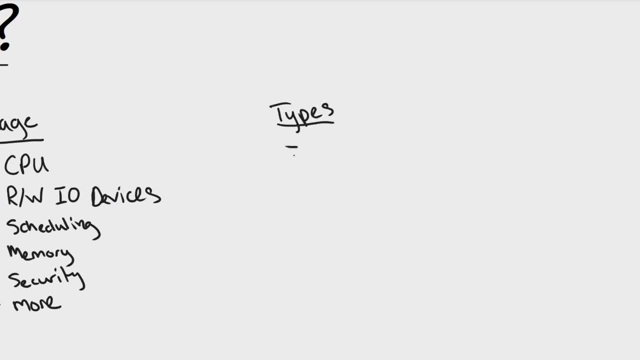 modules. Now that we talked about what is a kernel and what it does, let's talk about which kernels exist. I'm going to create another category called types. The first one is a monolithic kernel. Basically, with this one, the technology here is: if something gets hung up, it crashes the entire system, all due to the 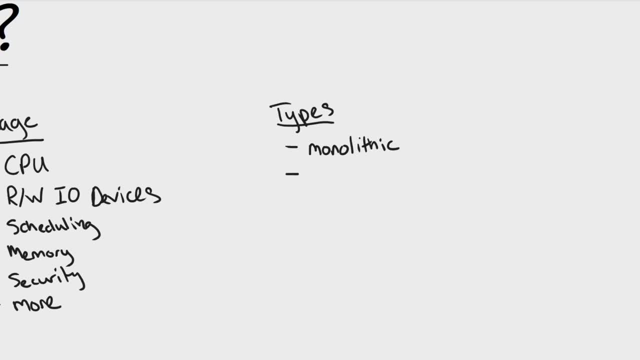 expense of speed. So if you want more speed, you would use a monolithic kernel, But of course you have to make sure that all your ducks are in a row or you can have a fatal system crash Again. this can make it faster than other kernels, but at the cost of having to be more stringent. 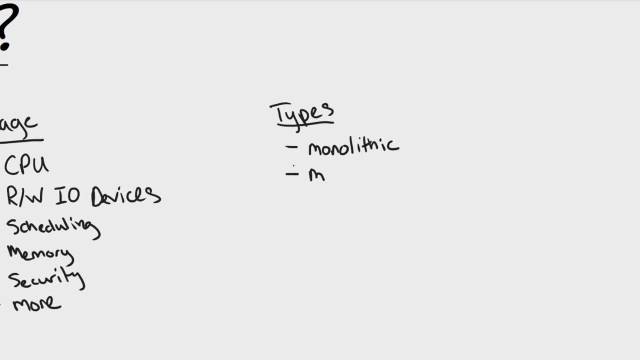 making it harder to manage. You also have a micro kernel here which takes on the opposite of a monolithic. Then we have an exo kernel. This one isn't used as much, so we won't talk about it- really Same as the rest of these we have. 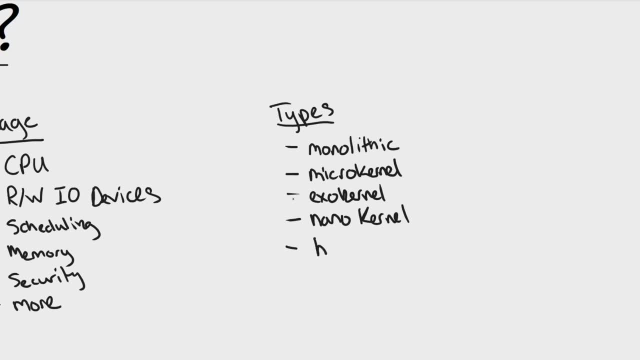 a nano kernel, and here probably the most popular one, is called a hybrid kernel, which is really just a mix between the monolithic and micro kernel. Most operating systems use a hybrid kernel type, and there is some debate in the kernel community whether or not hybrid kernel is even a thing, or if 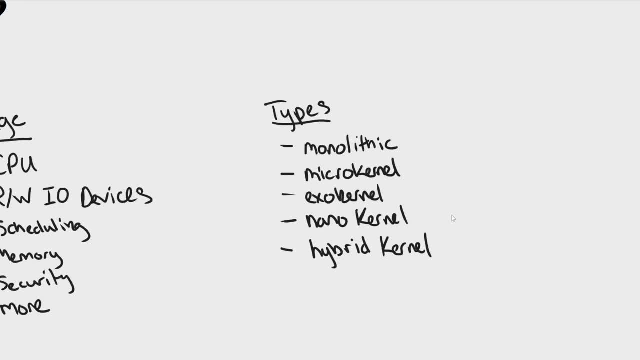 it's just a monolithic kernel that's handled properly. We'll let others debate that. Now that we understand the different types of kernel that we'd be making this way, we'll be making decisions aboutake dominance and mu ‑‑ thatئ. 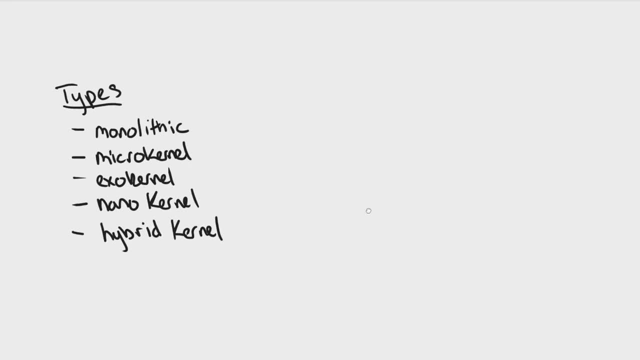 And now that we understand the different types of kernels, let's talk about the Linux kernel specifically. So the Linux kernel can be considered a monolithic kernel. It could also be probably considered a hybrid kernel, But again the debate's out on that for the terminology between monolithic and hybrid. 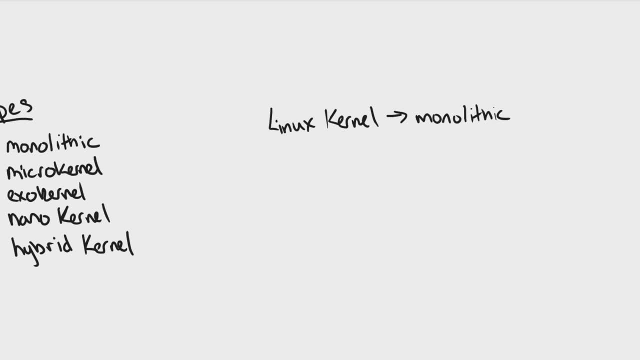 So I do believe that the Linux kernel calls itself a monolithic kernel. So then, if you ask yourself, Linux distributions and operating systems have to have a kernel which is called Linux. So what does Windows have? I'll give you a moment to take a guess.